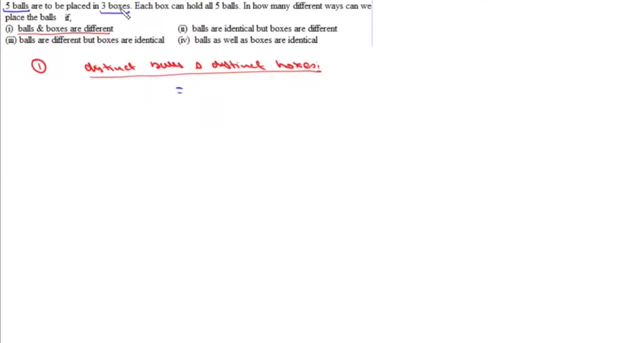 set B. Now, for this first ball we have three choices, So it can be put into any of the three boxes. So for the first ball we have three choices. For the second ball, we have three choices. For the second ball also, we have three choices, and it'll be the same for third, fourth and fifth ball. 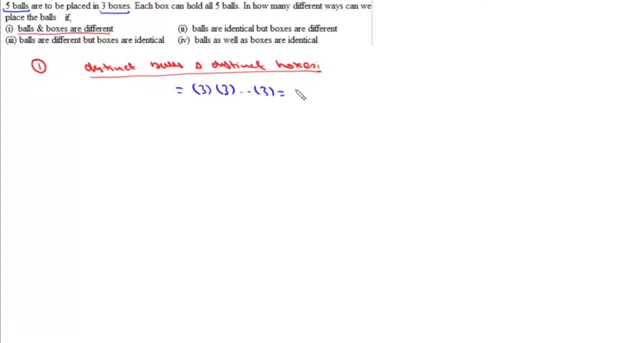 So total number of ways in which we can put five balls in three distinct boxes will be three to the power five. So if we take a general case where we have n balls, say B1, B2 and Bn, and we have r boxes- say B1, B2 and Br- then total number of ways in which we can put these 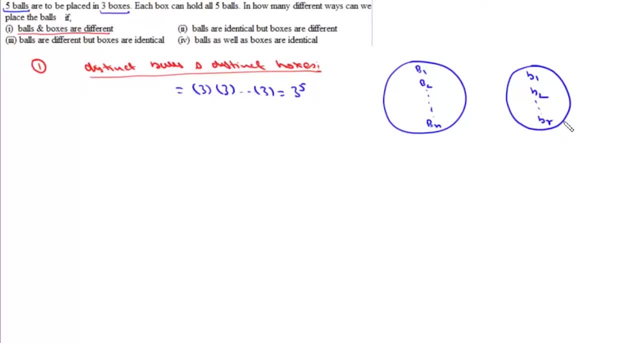 balls in boxes, when the balls and boxes both are distinct and the box can be empty. For this first ball, we have r choices. For second ball also, we have r choices. For this nth ball also, we have r choices. So total number of ways of putting. 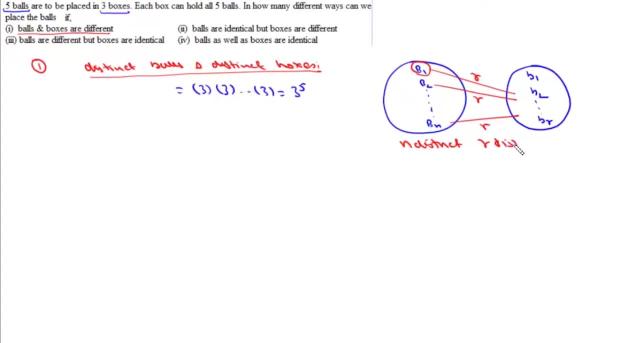 n distinct balls in r distinct boxes will be simply r into r into r n times and there'll be r to the power n. Now we'll consider the second case, when balls are identical but boxes are different, So we have identical balls in distinct boxes. 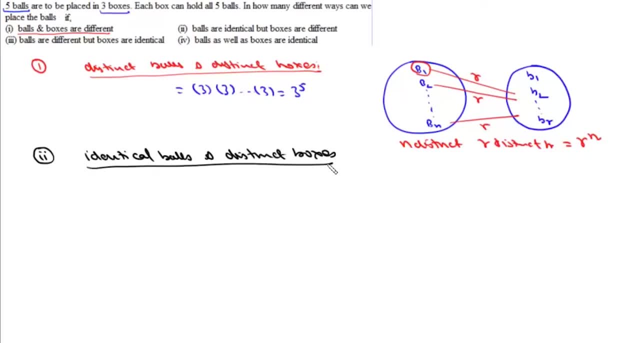 Now we got identical balls in distinct boxes- again our multi-set problem. but the balls are identical in boxes are distinct. We can use linear equations. So we have three boxes. Suppose number of balls and first box is x one, number of balls in second boxes x two and number of balls in third boxes x three. 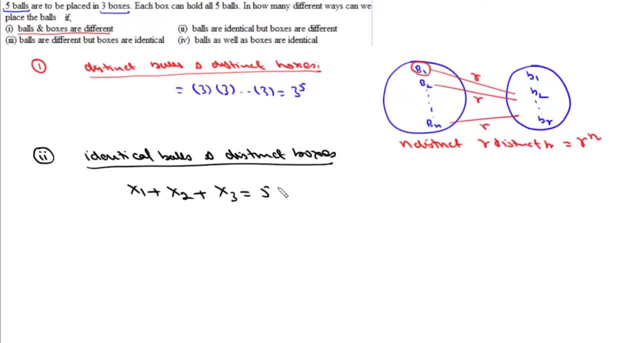 and total number of balls. It must be five. Now, any box can have any number of balls. So each of these x one, x two and x three. they must be greater than or equal to zero and they must be integer value. so we have to find. 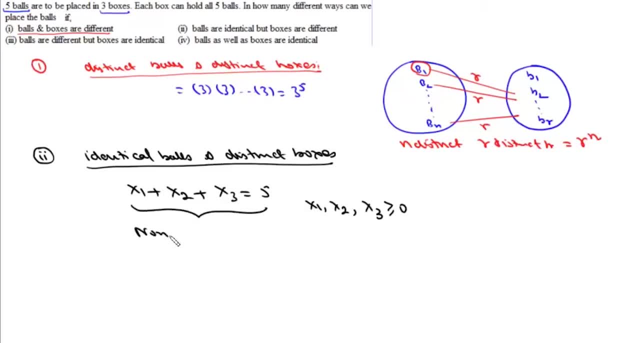 number of non-negative integral solutions. non-negative integral solutions now. previously, for the case when no box is empty, we have taken number of positive integral solutions. now here we are taking number of non-negative integral solutions, because here 0 is permitted. so number of non-negative integral solution in this case will be n, which is 5 plus r, r is 3 minus 1, c, r. 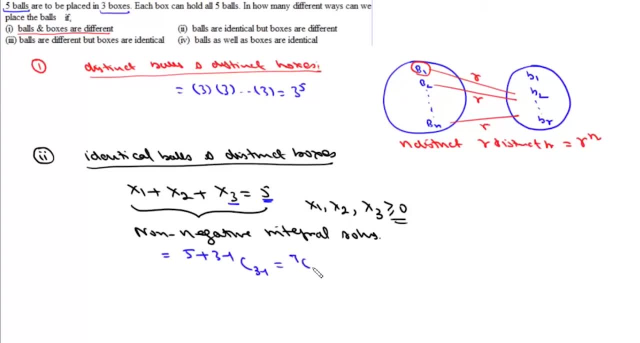 minus 1 and there will be 7 c 2.. now we'll take this general case. when we have n identical balls and r distinct boxes, then we can write this condition as this linear equation, which is x1 plus x2 plus xr, and it must be equal to n. 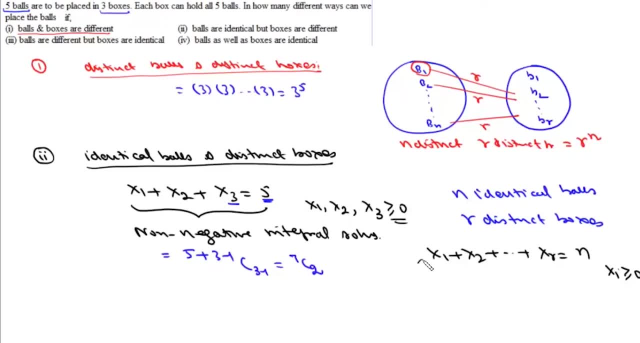 where each of xi is greater than equal to 0. we need to find number of non-negative integral solutions. so number of non-negative integral solution, number of non-negative integral solution in this case, is given by n plus r minus 1, c r minus 1. so this is how we distribute identical. 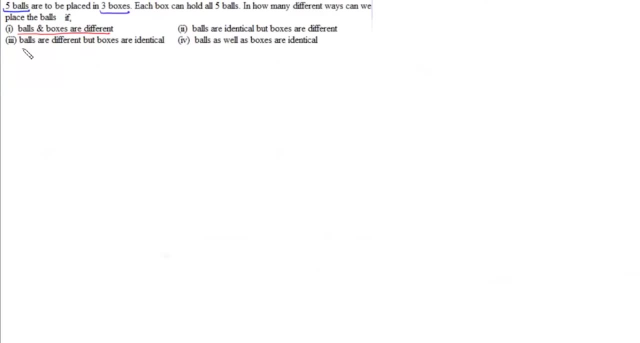 boxes. now we'll take up this third case, when balls are different but boxes are identical. so here we have five distinct balls and three identical boxes. now how can we distribute these distinct balls in identical boxes? now, since it has distinct balls, it is a distribution problem. so we'll consider three cases. case one, when all the five balls 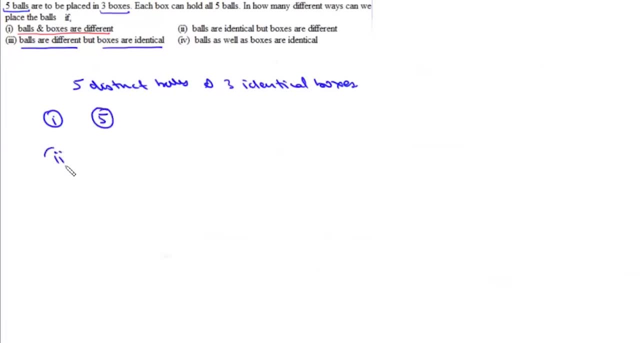 they're distributed in only one box. second case, when these five balls are distributed in two boxes. in two non-empty boxes they can be distributed as either 4: 1 or 3: 2. and this third case, when all these five balls they are distributed in three non-empty boxes, so it 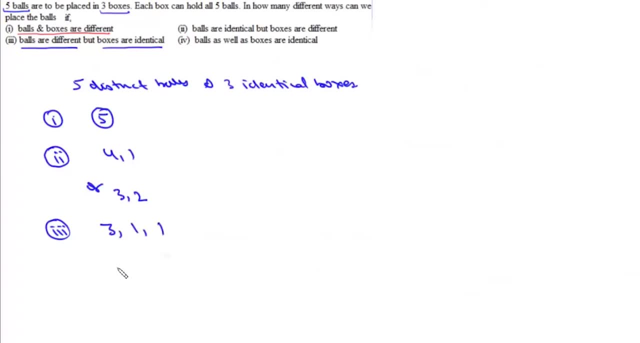 can be done in either 3, 1 one way, or 2, 2 and one way. now for this first case. from these five we need to select five and it can be done in only one way. now for this second case, we have to distribute this five in two groups containing four and one, so it'll be factorial five divided by factorial. 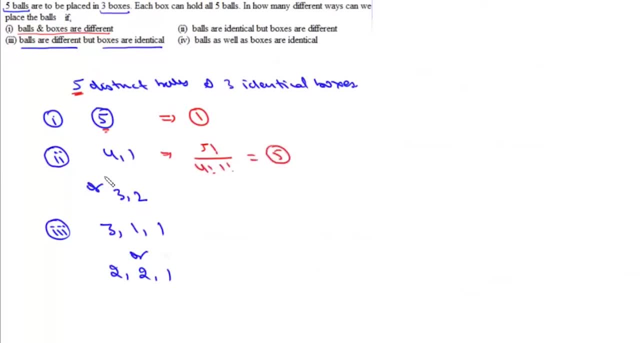 four, factorial one, and it'll be simply five. then we have to distribute this five in groups of three and two. it'll be factorial five, factorial three, factorial two, and it'll be simply ten. now, what about three? one, one. it'll be factorial five, factorial three. factorial one, factorial one. 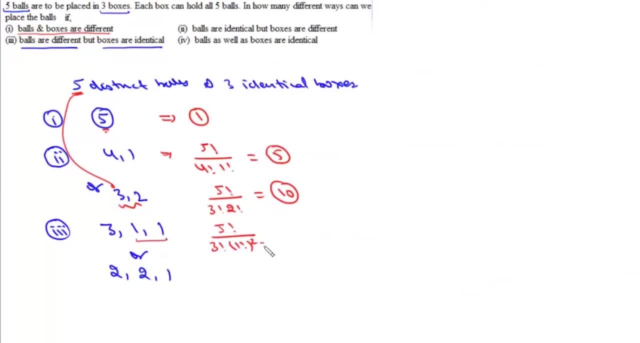 whole square. and then, since these two numbers, they are same, so we have to divide it by factorial two, so it'll again be 10, and here it will be factorial 5, factorial 2, square, factorial 1, and again we have two numbers same, so divide by factorial 2, so it'll be 15.. so we'll add them. 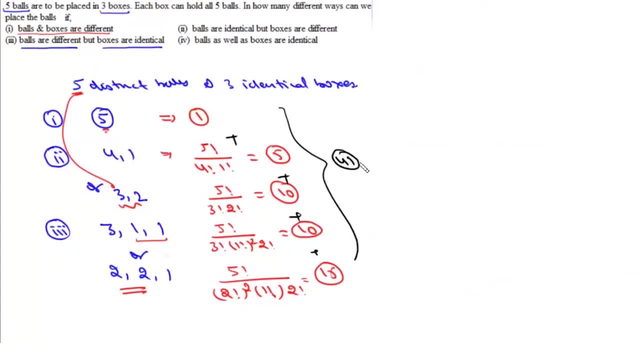 total number of ways will be simply 41, so there will be 41 ways in which we can distribute these five distinct balls in three identical boxes. so, essentially, what you have done is we have used the same formula of distributing distinct balls in boxes if no box is empty. 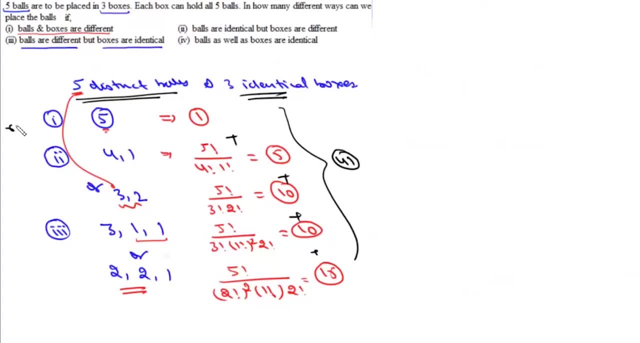 considering we have to distribute the same number of balls in the same number of boxes three separate cases: when we have only one box, when we have two boxes and when we have three boxes. so general case of solving this problem will be: suppose we have n distinct balls and we have are identical boxes. then number of ways of distributing n distinct balls in 3 separate cases. 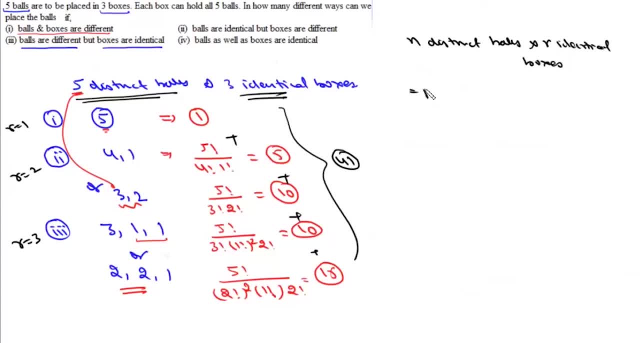 in R, identical boxes will be given by this Bell number, BN, and which is nothing but sum of the Sterling's number of second kind, S, NK, where K varies from 0 to R. So for this case we'll need to find this summation: K varies from 0 to 3 S. 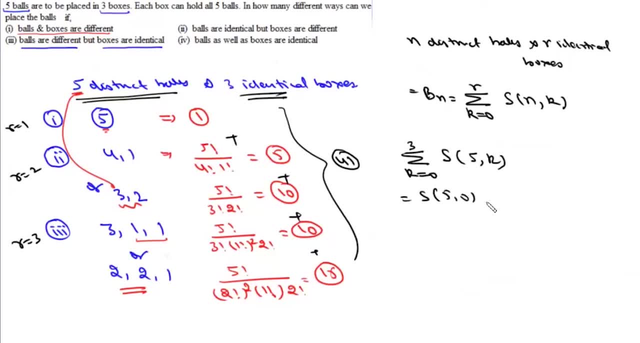 5 K, which is S 5 0 plus S 5 1 plus S 5 2 plus S 5 3.. Now S 5 0, it is 0, S 5 1 is 1, S 5 2 is 15 and S 5 3 is 25.. 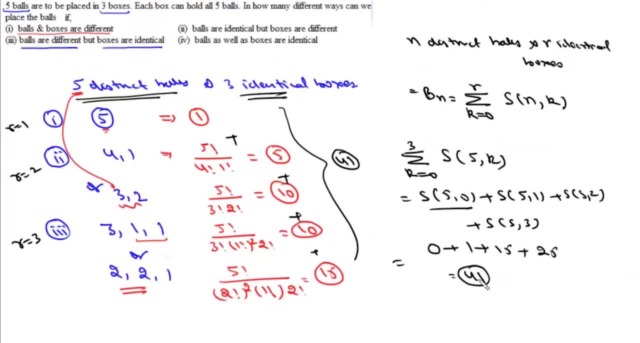 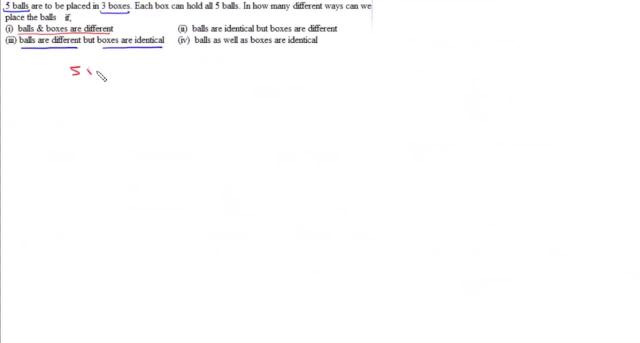 So this value? it again comes out to be 41.. And finally, we have this case when balls as well as boxes are identical. So here we have five identical balls and three identical boxes. Now these five identical balls are to be distributed in three identical boxes. 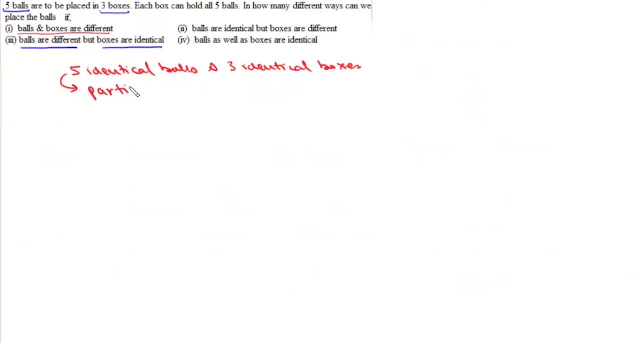 Now this again is nothing but a partition problem. So previously we have partitioned five and three sets, all three sets Now, since in this case empty boxes are allowed. So we need to find this partition: P5, one plus P5, two plus P5. 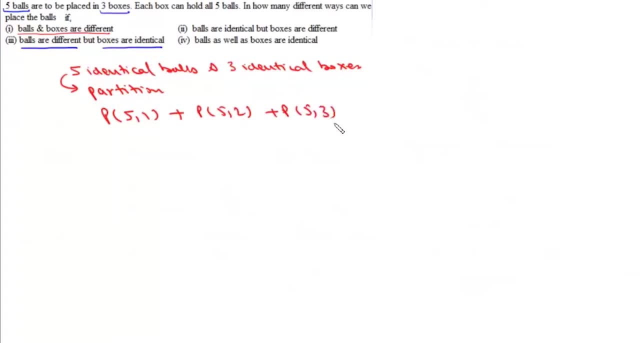 So if no box is empty, then we just have to find P5 three. But here we have to find P5, one plus P5, two plus P5 three. Now, in how many ways we can partition five and one? so there is only one way. 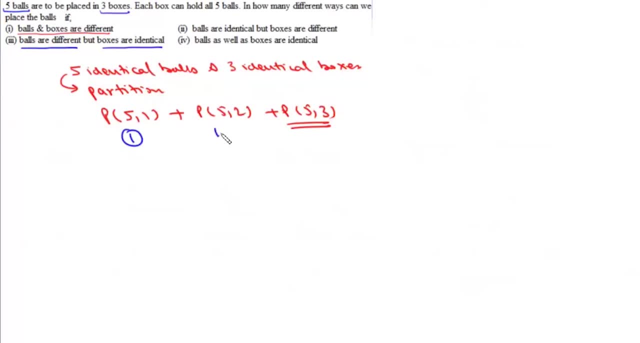 Now, what about five and two? Now, five and two can be either 1 plus 4, 5 and 2.. So there is only one way. Now, what about 5 and 2?? Now, 5 and 2 can be either 1 plus 4, 5 and 2.. 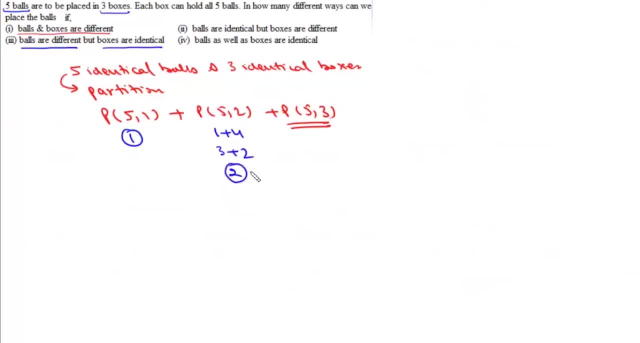 or three plus two. So there'll be two ways, and five and three will be one plus one plus three or two plus two plus one. So we have two ways here. So total number of ways will be simply five. So we can distribute five identical balls in three identical boxes in. 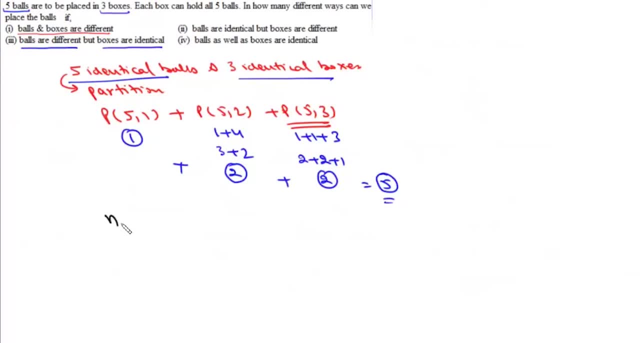 five ways. We have to write its general formula. So we have n identical balls and r identical boxes. Then all we need to do is we need to find this p n k, where k varies from one to r. So we have to find some of these partitions, p n k. Now for our problem.